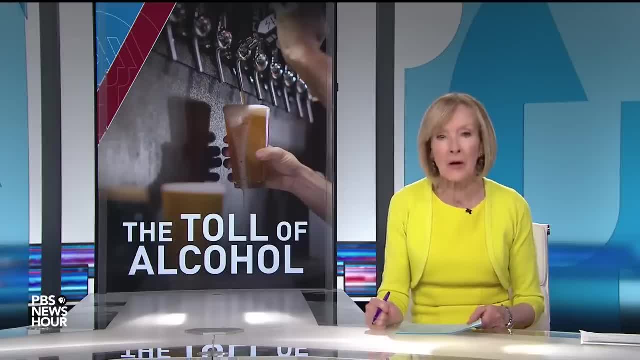 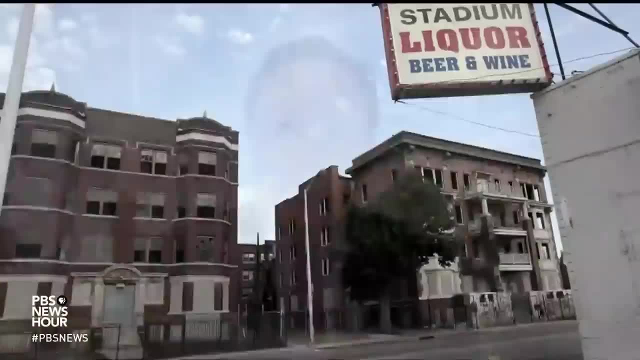 A new study documents just how big a toll it is taking on American lives. John Yang has the details. JOHN YANG, The New Yorker" Judy. the study, which is from the Centers for Disease Control and Prevention, found that between 2015 and 2019, one in eight working-age Americans 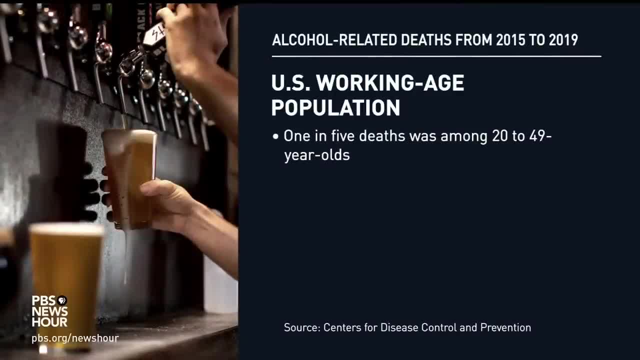 died from excessive drinking. Among those ages 20 to 49, one in five deaths was attributable to alcohol. For those ages 20 to 34, it was one in four. Overall, working-age Americans accounted for nearly two-thirds of the nation's annual average. 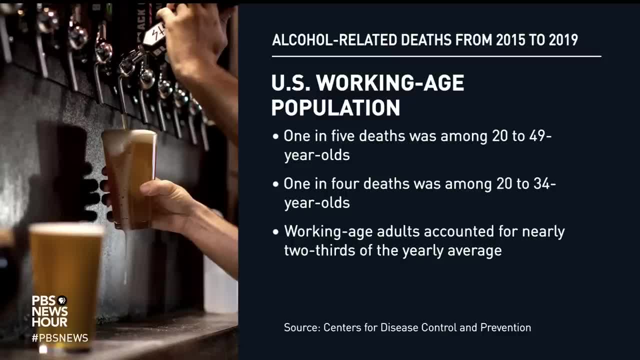 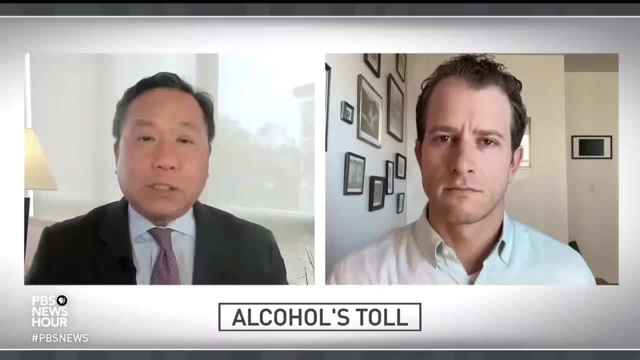 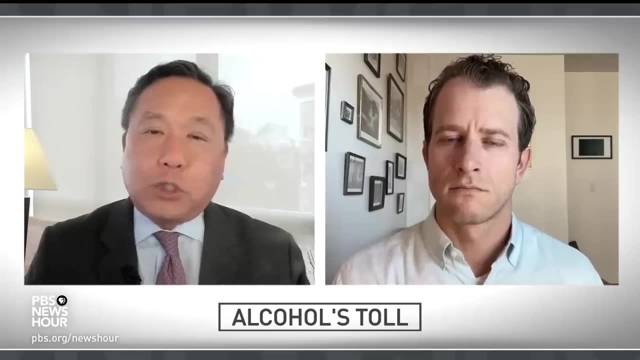 of 140,000 alcohol-related deaths. Ted Alcorn is an independent journalist who covers health and justice for The New York Times and other outlets. Ted, thanks so much for joining us. I know you watch this issue very, very closely. What struck you or what stood out to you from? 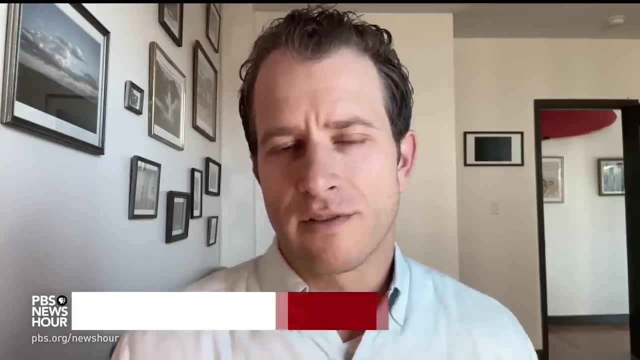 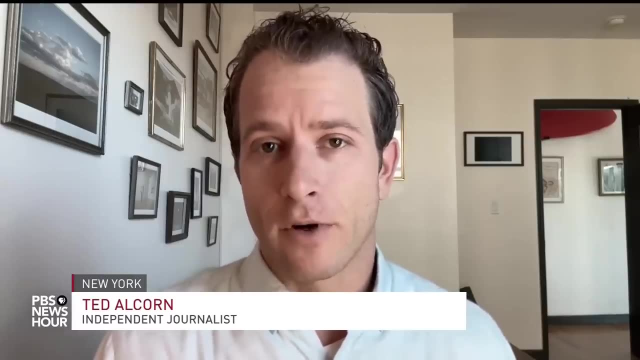 this report, TED ALCORN, The New Yorker" Well, the CDC only do this kind of analysis and release this full accounting of alcohol-related deaths every few years, And the trends have been going up for a long time. but it's still shocking, when you see it, that alcohol is killing about. 140,000 Americans a year, and two-thirds of those deaths are people in their working age, from 20 to 64. So it's not only a huge public health problem, but it's cutting to the core of people in the prime of their life, when they're economically productive. And for all those reasons it's. 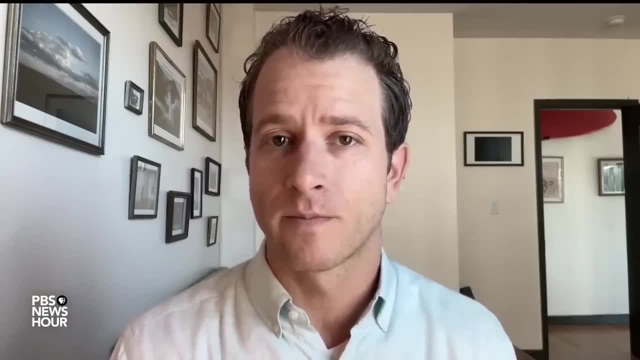 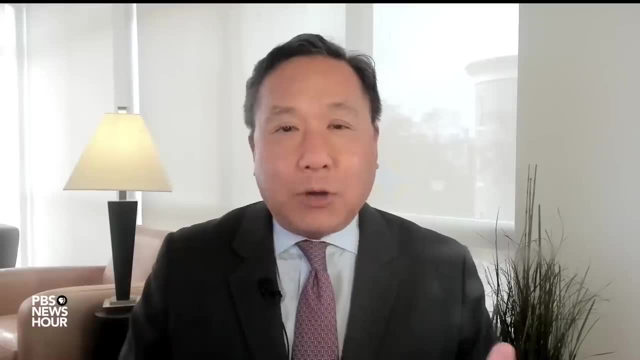 a little bit neglected as a public health crisis in this country. JOHN YANG, The New Yorker" You talk about sort of neglected as a public health crisis. So much attention has been given to opioids in the recent years. Can you compare the two? 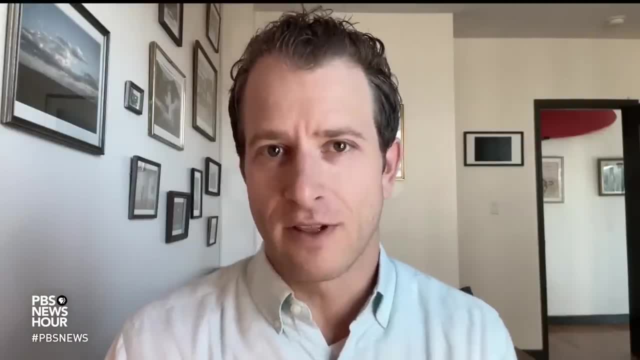 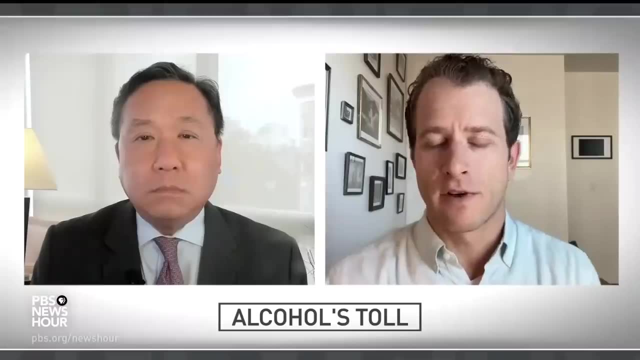 TED ALCORN, The New Yorker" Well, clearly the country's been juggling a lot of public health challenges for the last few years. We have our plate full for sure, And we're rightly given a lot of attention to opioid overdose deaths, which 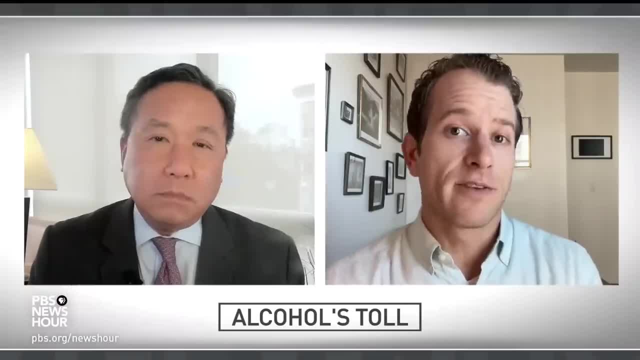 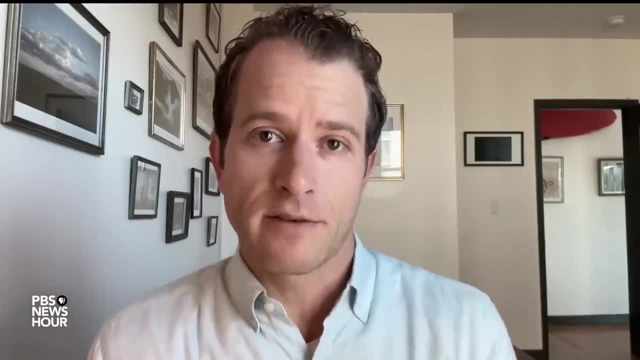 have been climbing. I have done a lot of reporting on that as well, But those deaths come to around 100,000 people a year. So, as you can see, alcohol actually kills more people than opioids, but gets, I would say, a fraction of the attention. 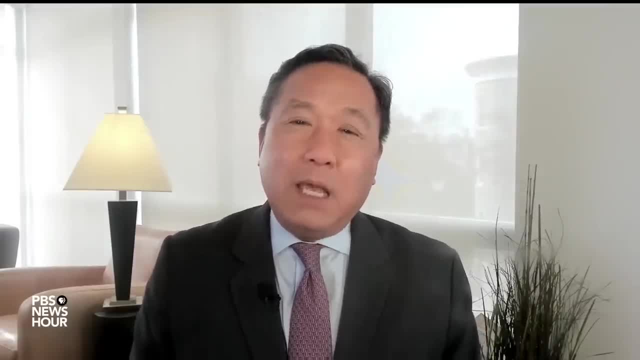 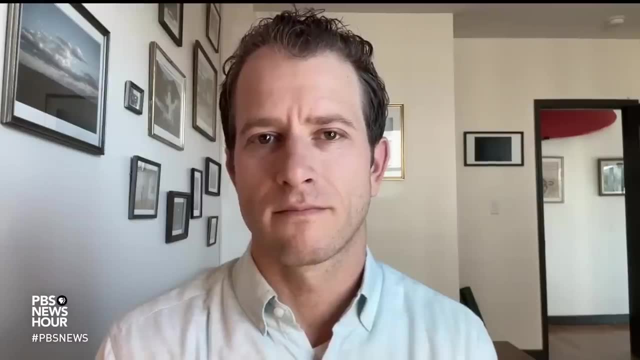 JOHN YANG, The New Yorker". Why doesn't it get as much attention? I mean, this is a substance that's largely legal, is sort of lightly regulated In a lot of ways compared to opioids. does that sort of create this impression that it's? 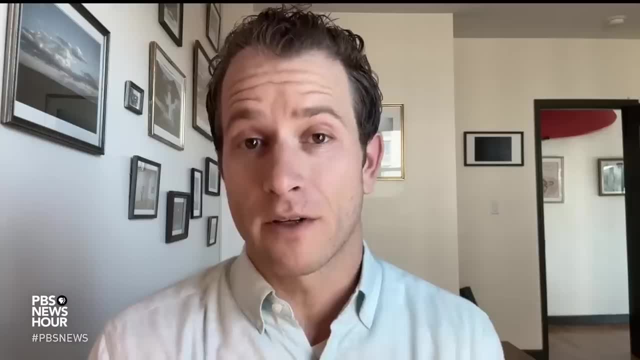 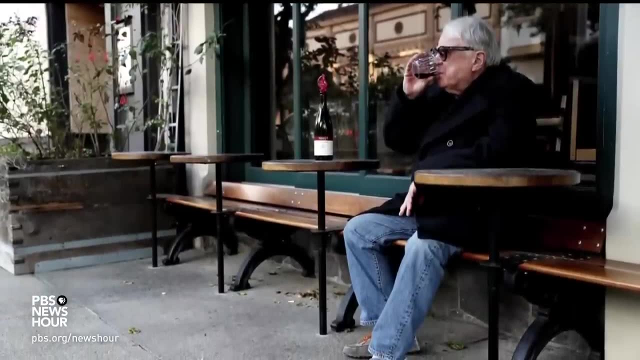 not a problem. TED ALCORN, The New Yorker". Well, alcohol is a popular commodity. It's still a minority of Americans that actually partake, but that amounts to tens of millions of people who enjoy it responsibly And it's a part of meaningful happy moments in a lot of our lives, But it 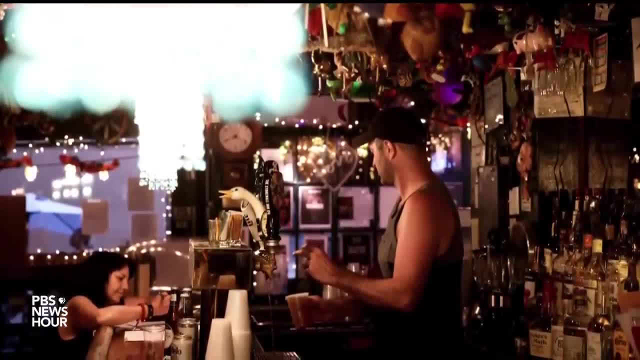 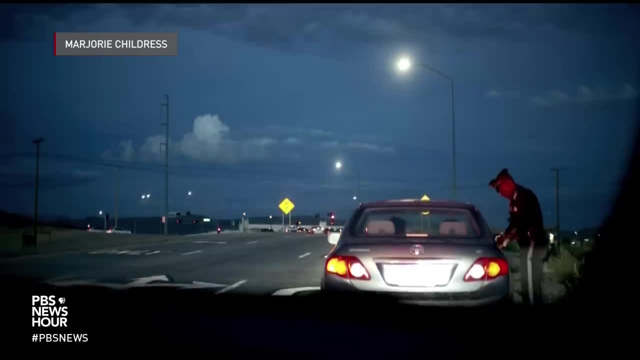 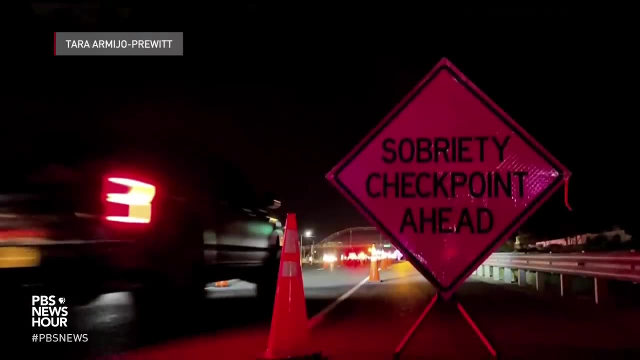 also has huge societal costs, And I think we underappreciate those harms because some of them are scattered across the health system- I think of alcohol and its impacts being on the roadways in terms of drunk driving accidents- and don't recognize the huge number of chronic disease deaths that it contributes. 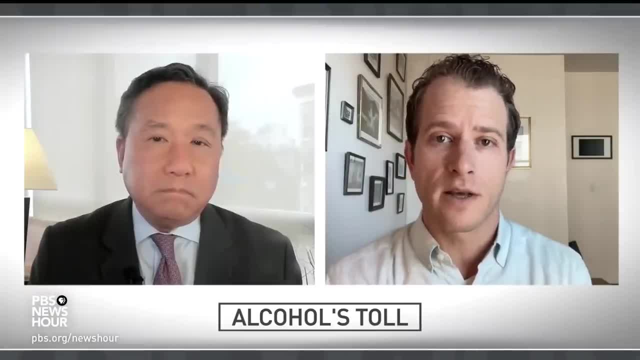 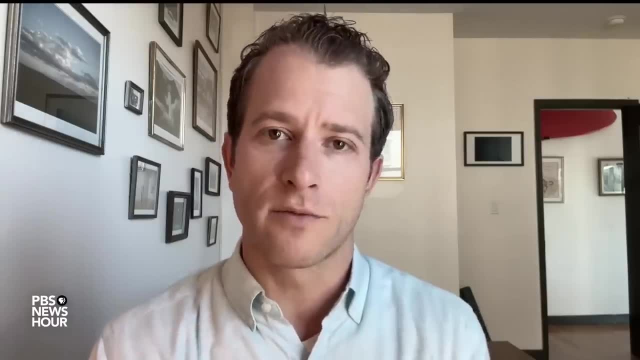 to The CDC study put together 58 different causes of death. All are alcohol attributable, including some that aren't necessarily top of mind of people but are very important. Alcohol is a risk factor for breast cancer among women. It's actually now thought to contribute to. 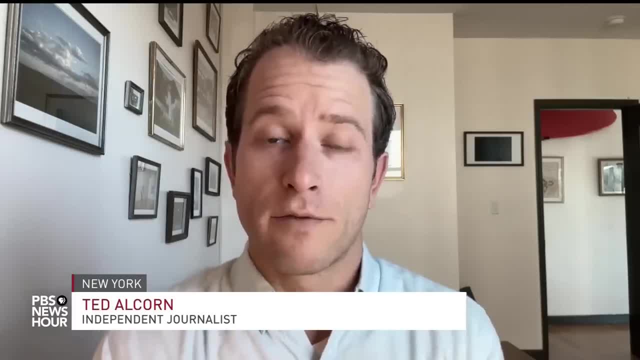 cardiovascular disease. So, for all those reasons, only when, with CDC, we're able to do that. JOHN YANG The New Yorker". So you know, I think it's important to think of alcohol and its impacts being on the roadways in terms of drunk driving accidents, and don't recognize 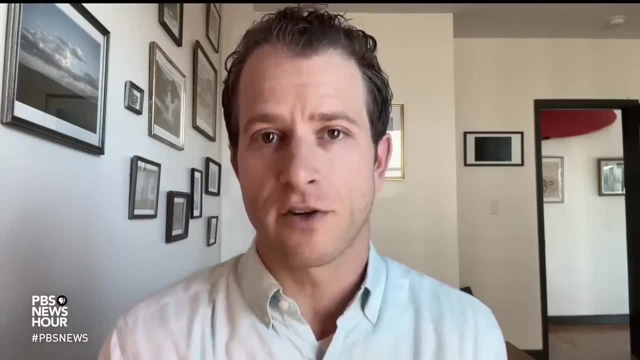 those harms. But when the CDC puts all of these causes of death together, do we really get a full picture of the catastrophic damage it's doing? JOHN YANG, The New Yorker". And the data in this study only goes up to 2019, because 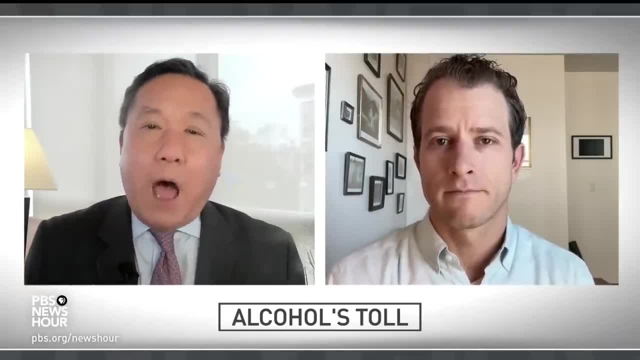 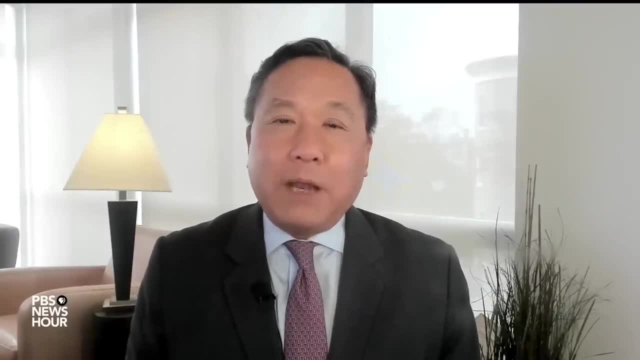 of how they collect the data and that sort of thing, Obviously before the pandemic, During the pandemic, with social isolation, is there any sense that this might have actually gotten worse? JOHN YANG, The New Yorker" The data that the CDC puts together in this comprehensive 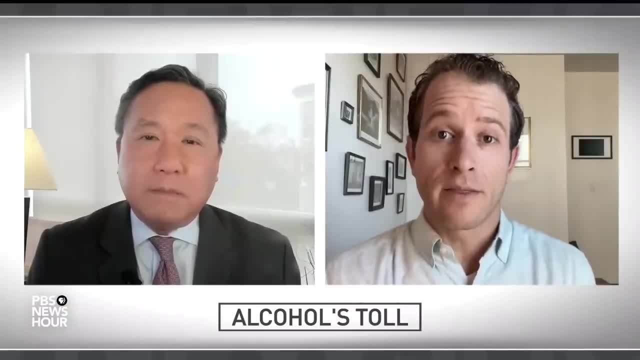 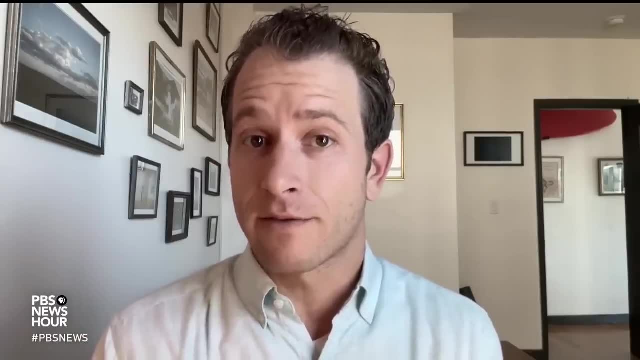 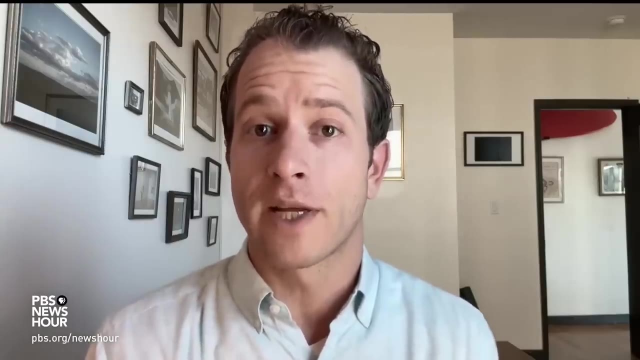 way is, as you point out, already a few years out of date, But the preliminary data mortality that we have from 2020 suggests that, indeed, some kinds of alcohol-related deaths jumped considerably that year, And it was a period of time when people appear to have been drinking. 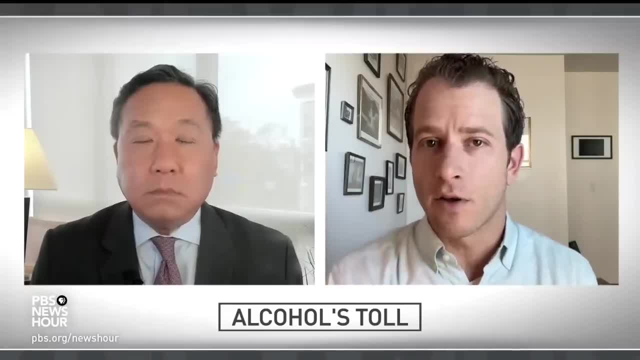 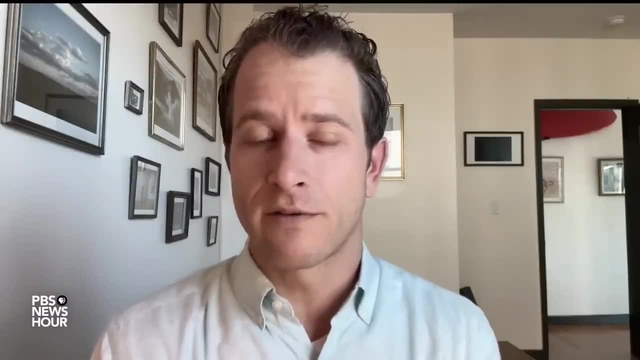 more frequently drinking at home and drinking sometimes at a higher volume than they would have been if they'd been out at restaurants or bars. So the numbers as they come in now for this year and in future years are likely to be even worse. 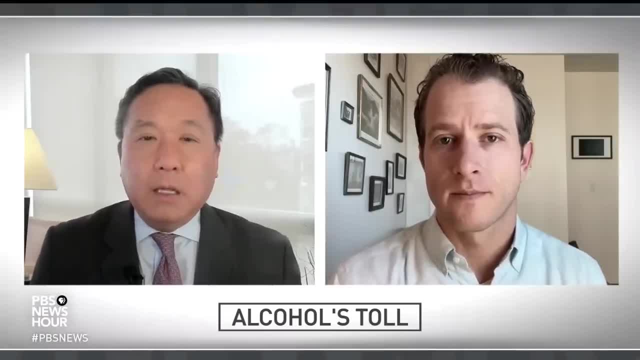 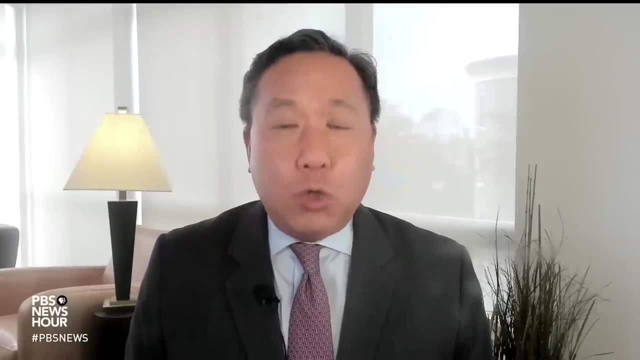 JOHN YANG, The New Yorker". The study also showed wide disparity in deaths- Alcohol-related deaths, from region to region. for instance, in New Mexico it's incredibly high. You looked at New Mexico. What's going on there? Why is it so high there?